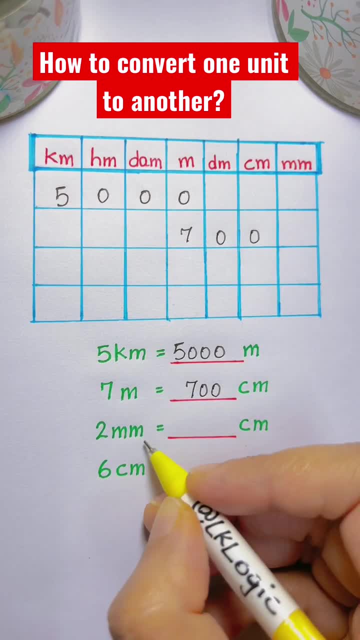 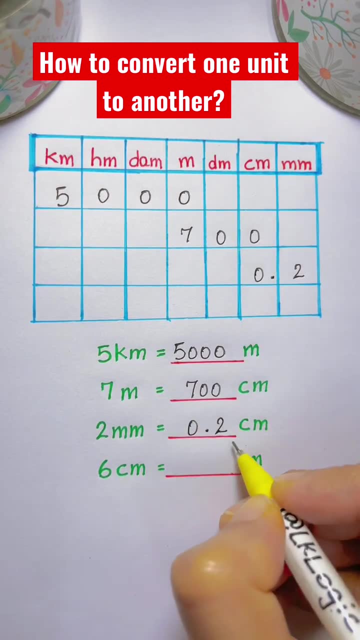 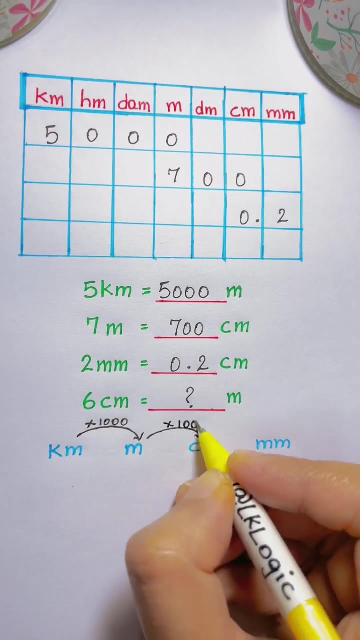 centimeters, so fill up with zero. seven hundred centimeters. two millimeters, two centimeters, so just put a two under millimeters and 0.2 centimeters. so what is this? so, basically, when you're converting a larger unit to a smaller one, you multiply by the multiples of 10 and 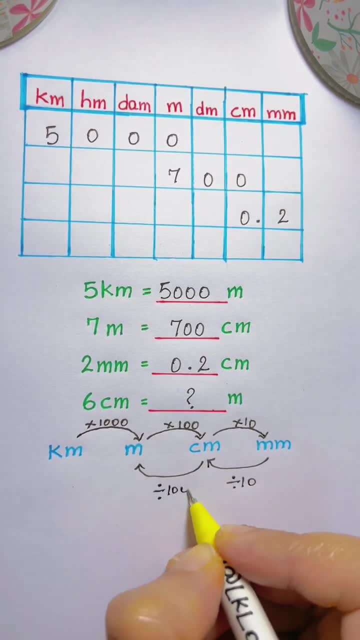 when you're converting a smaller unit to a larger one, you divide by the multiples of 10. 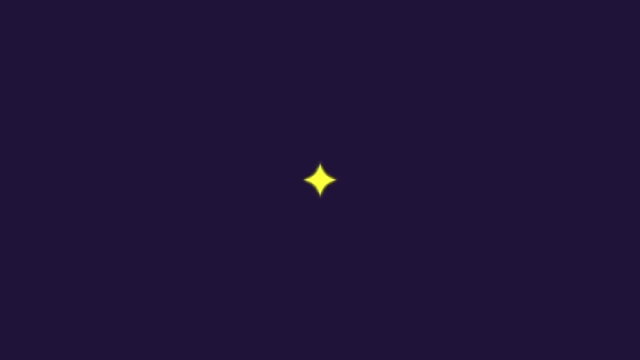 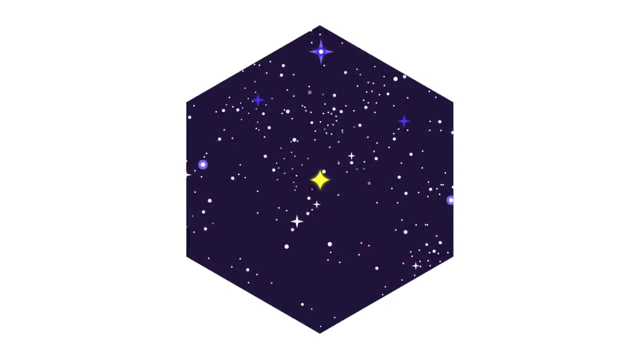 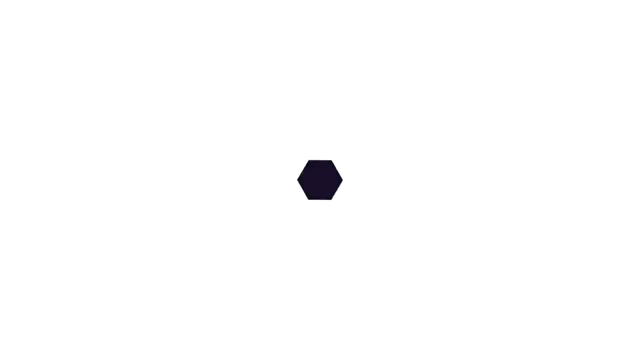 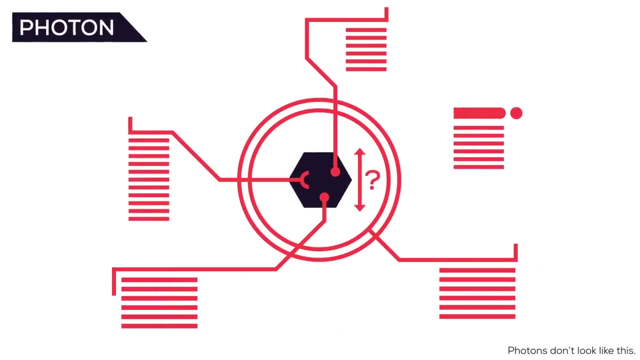 Light is the connection between us and the universe. Through light we can experience distant stars and look back at the beginning of existence itself. But what is light? In a nutshell? light is the smallest quantity of energy that can be transported: A photon, an elementary particle without a real size, that can't be split, only created or destroyed. 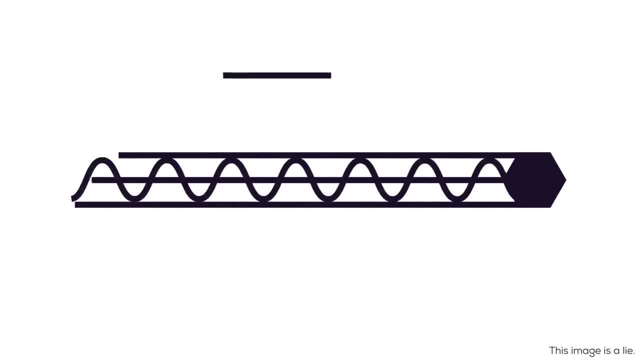 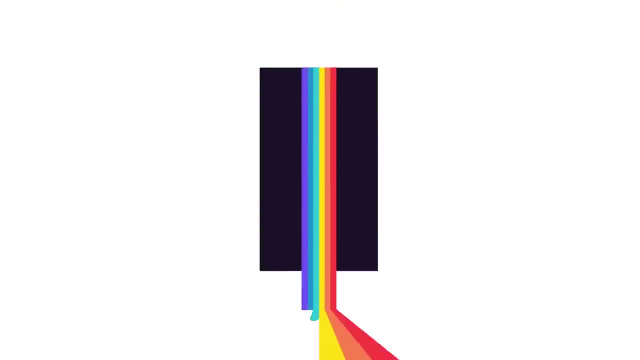 Light also has a wave-particle duality, being kind of a particle and a wave at the same time, although this is a lie. Also, when we say light, we actually mean visible light, which is a tiny part of the electromagnetic spectrum, energy in form of electromagnetic radiation. 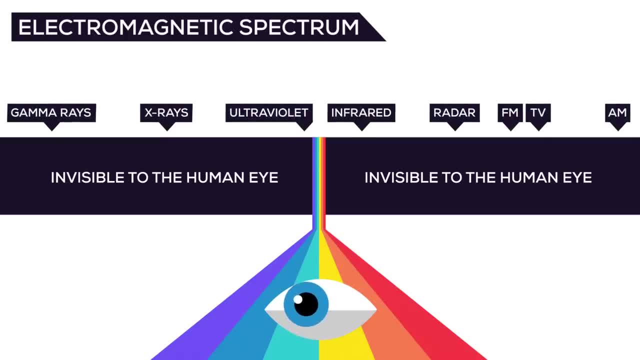 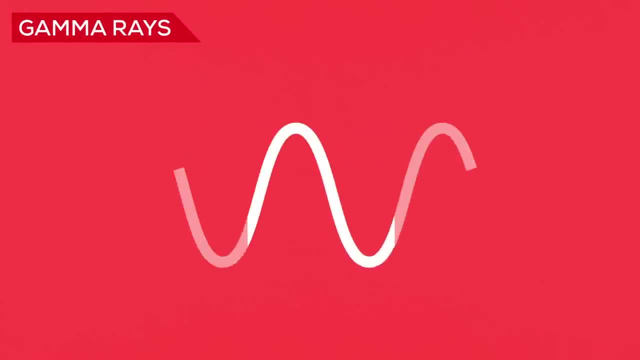 Electromagnetic radiation consists of an enormous range of wavelengths and frequencies. Gamma rays have the smallest wavelength Because they're the highest energy photons, But most gamma rays are just under 10 picometers, which is still way smaller than a hydrogen atom. 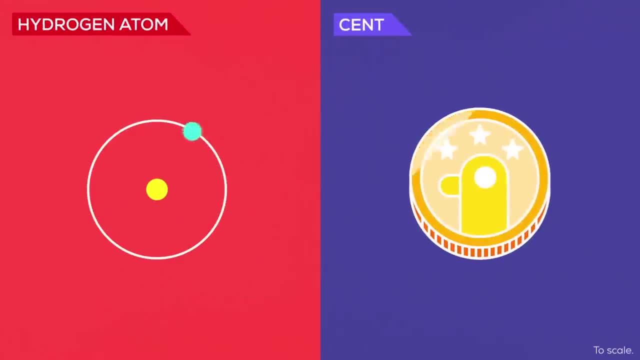 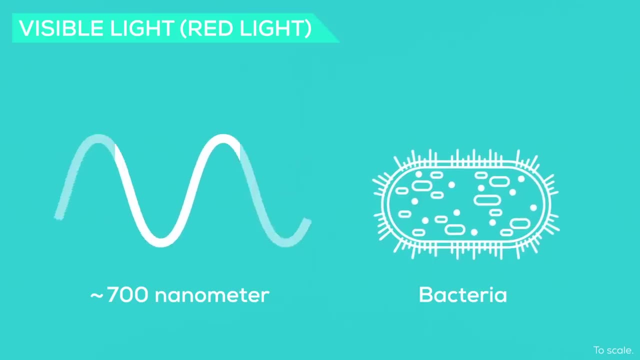 For reference, a hydrogen atom, compared to a cent, is about as big as a cent compared to the moon. Visible light is in the middle of the spectrum in the range of about 400 nanometers to 700 nanometers, about the size of bacteria. 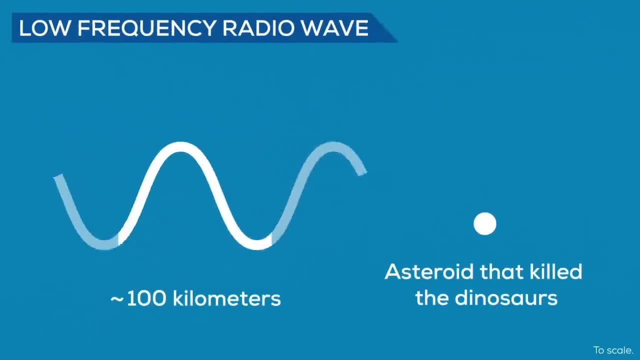 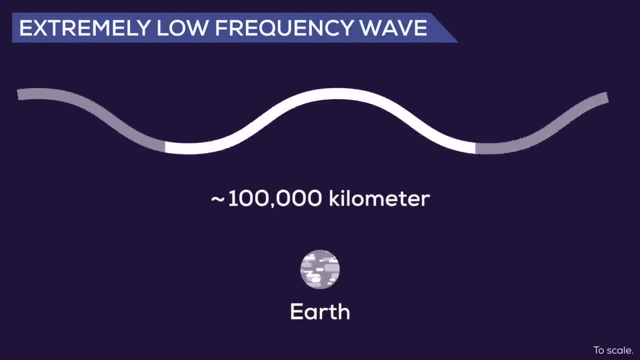 On the other end of the spectrum, radio waves can be up to 100 kilometers in diameter, While the biggest wavelengths we know exist can span for thousands of kilometers, From 10,000 kilometers to a baffling 100,000 kilometers, way larger than Earth.